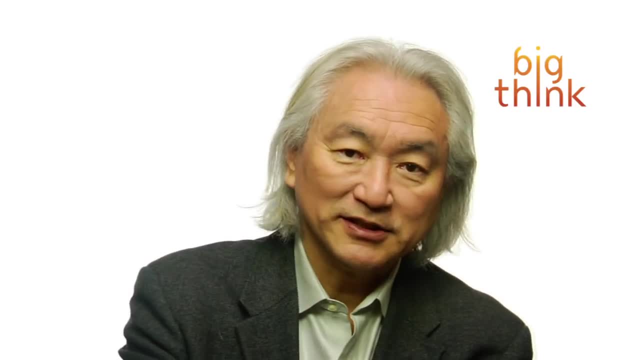 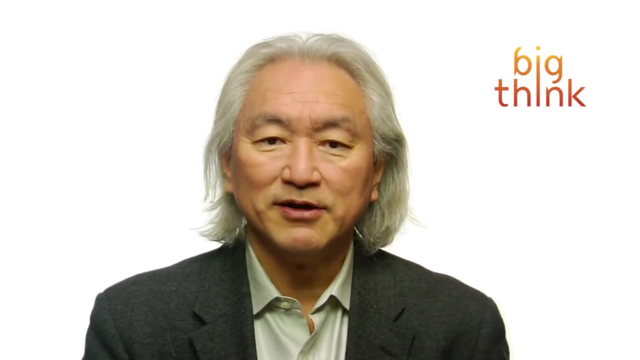 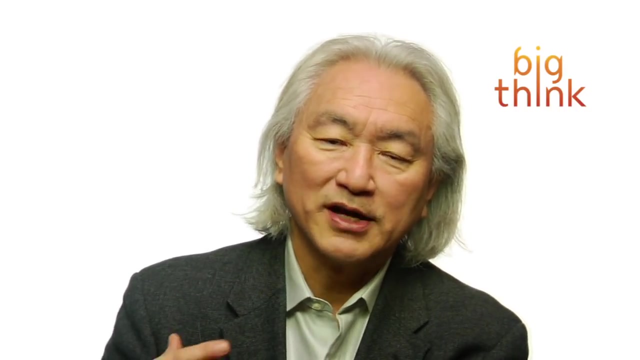 strings and membranes obeying the laws of physics, which is nothing but the laws of harmony of vibrating strings. But why 11?? It turns out that if you write a theory in 15,, 17,, 18 dimensions, the theory is unstable. It has what are called anomalies, It has singularities. It turns out that mathematics 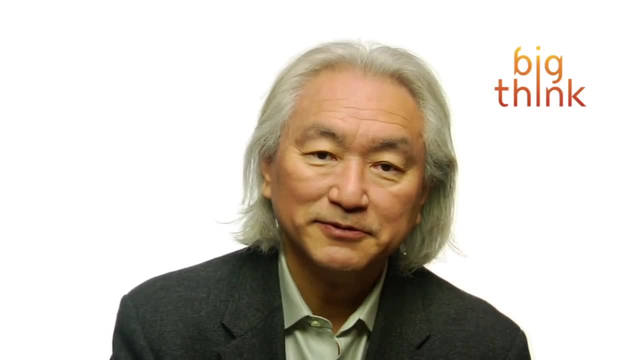 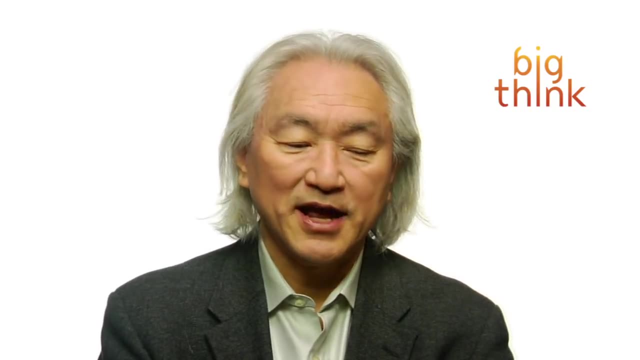 alone prefers the universe being 11 dimensions. Now some people have toyed with 12 dimensions. At Harvard University, for example. some of the physicists there have shown that a 12-dimensional theory actually looks very similar to an 11-dimensional theory. 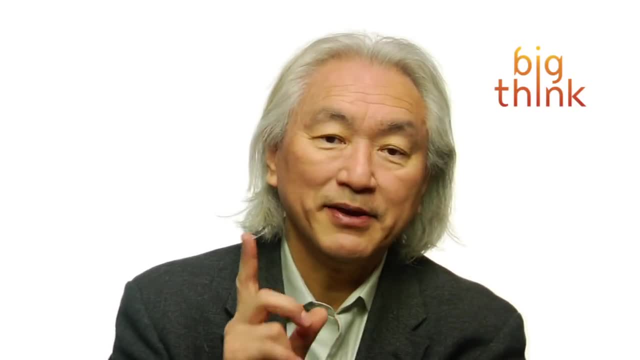 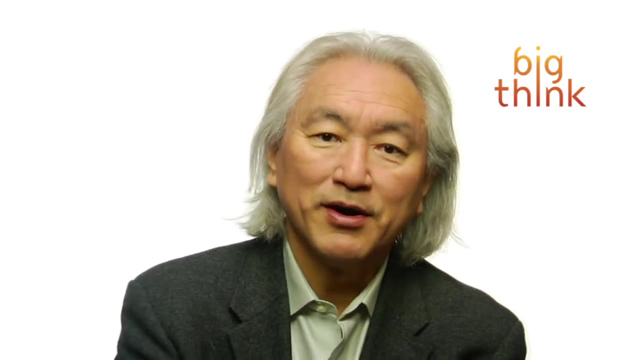 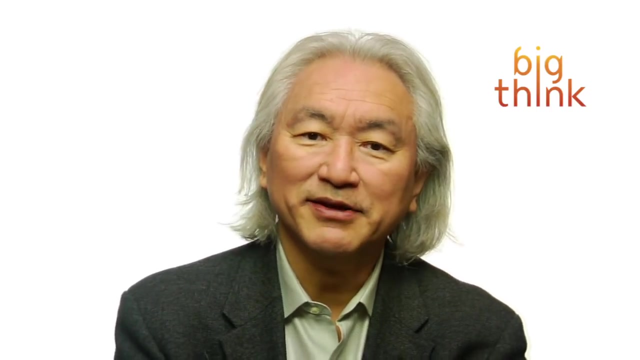 But why 11?? Why 11?? Why 11?? That's because the rule of law is not every 11 dimensional theory, except it has two times, double times, rather than one single time parameter. Now, what would it be like to live in a universe with double time? Well, I remember a movie with David Niven. David Niven played 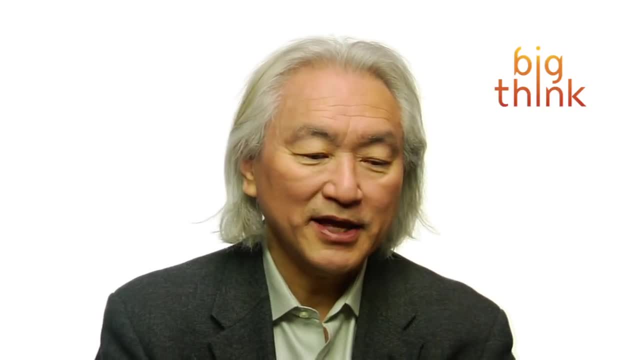 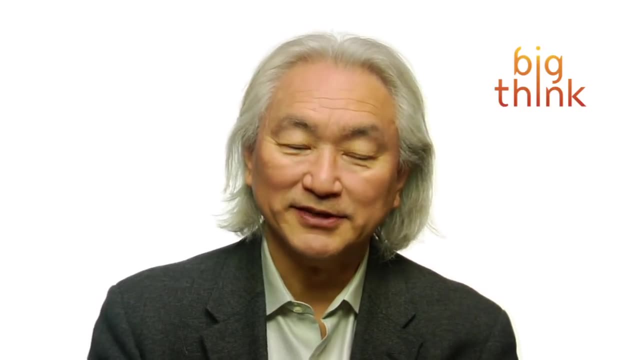 a pilot who was shot down over the Pacific. But the angels made a mistake. He was not supposed to die that day, And so the angels brought him back to life and said: oh, sorry about that, killed you off by accident. you were not supposed to die today. 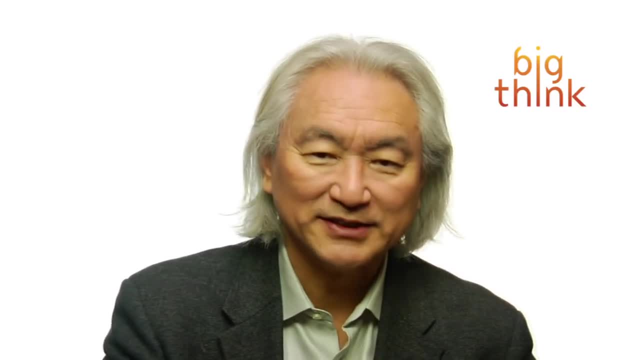 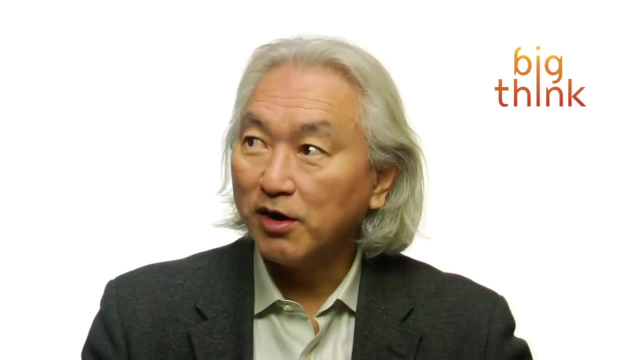 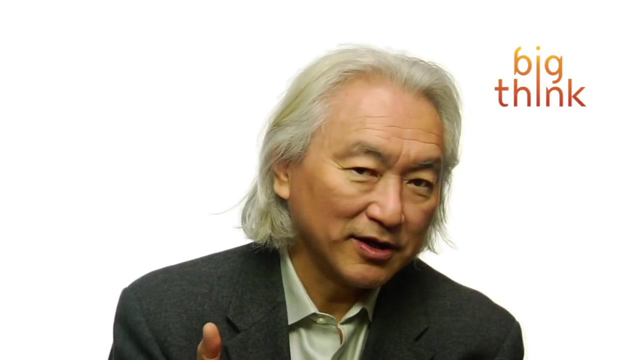 So in a great scene, David Niven then walks through a city where time has stopped. Everyone looks like this And there's David Niven just wandering around looking at all these people. That's a world with double time. David Niven has one clock, but everyone else has a separate clock, and these two clocks 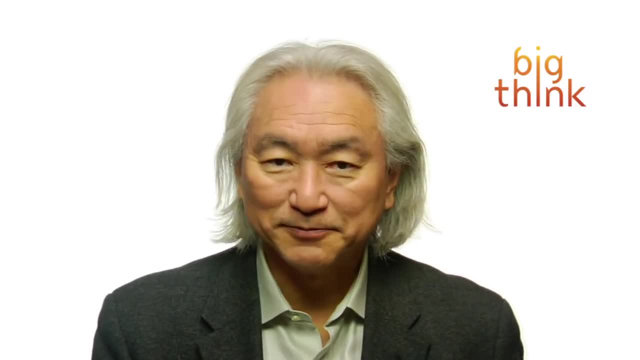 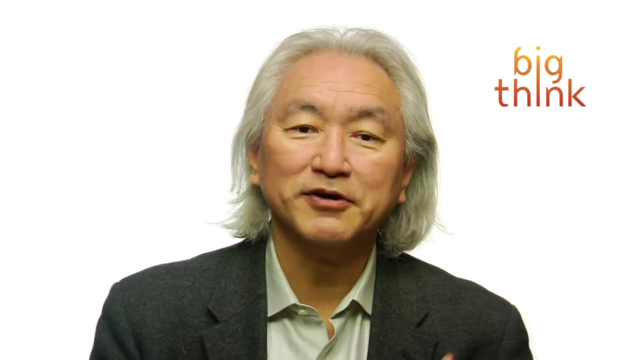 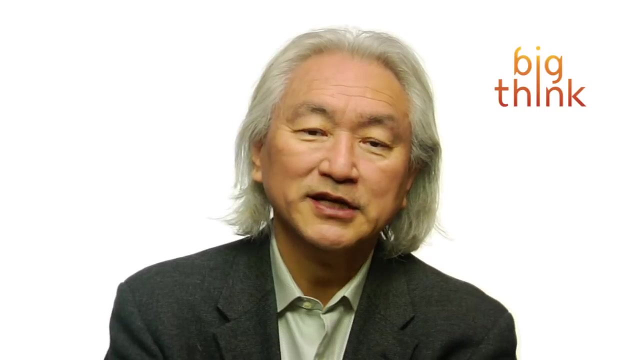 are perpendicular to each other. So if there's a double time universe, you could walk right into a room, see people frozen in time while you beat to a different clock. That's a double time universe. Now, this is called F-theory, F for father, the father of strings. It's not known whether F-theory will survive or not. however, M-theory in 11 dimension is the mother of all strings and that theory works perfectly fine. So, to answer your question, in other dimensions- Dimensions beyond 11,, we have problems with stability. 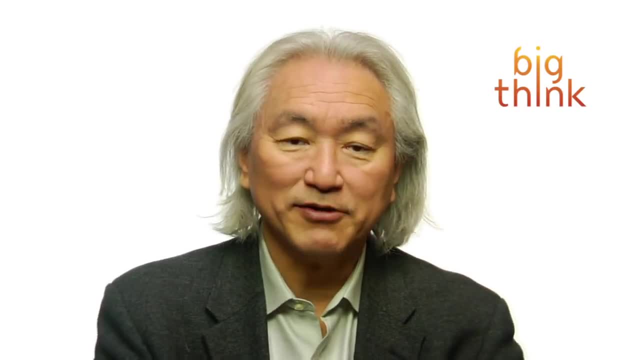 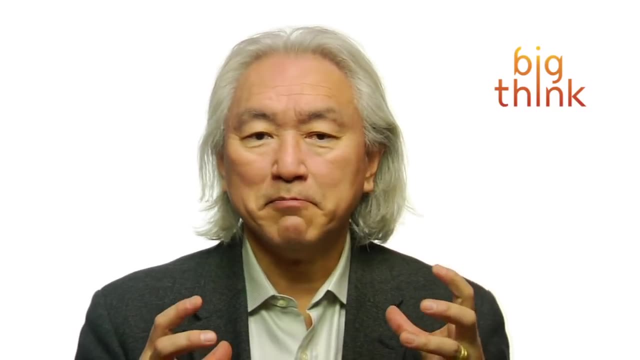 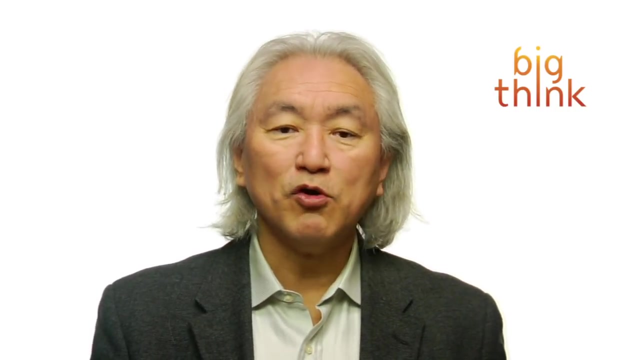 These theories are unstable. They decay back down to 11 dimensions. They have what are called anomalies, singularities which kill an ordinary theory. So the mathematics itself forces you to 11 dimensions. Also, because this is the theory of everything, there's more room in higher dimensions to put all the forces together. When you put gravity, electromagnetism and the nuclear force together, 4 dimensions is not big enough to accommodate all these forces. When you expand to 11 dimensions, bingo- everything forms perfectly well.